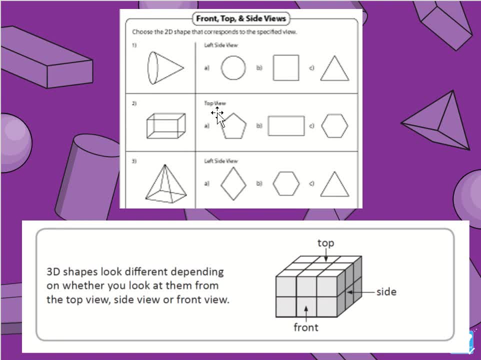 Now let us have a look at this prism. If we were looking at it from a top view and we were looking down, what shape would we see? Would it be a pentagon, a rectangle or a hexagon? Now, I would pick the rectangle, because that is the shape that I would see if I was looking. 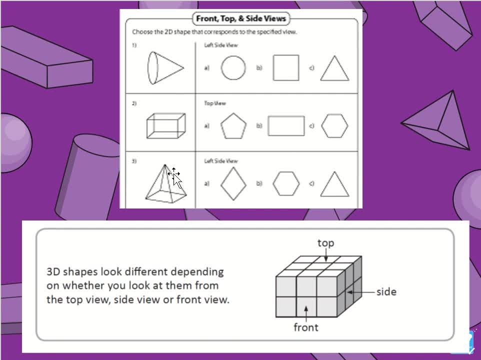 at it down or from the top. Now let us have a look at this. This is a pyramid and it is asking: what would it look like from the left side? Would it be a diamond, a hexagon or a triangle? Which one would it be if you were looking at it from a side view? So, not the 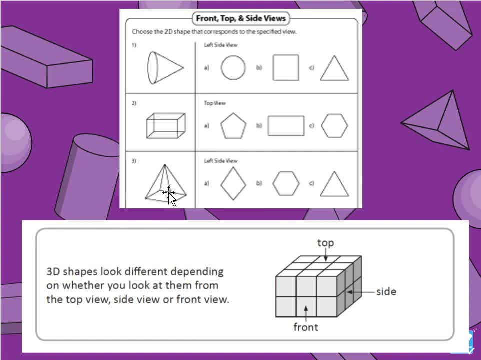 top view, Not the bottom view or the front. So this is the left. the left side It would be a triangle. Okay, so 3D shapes look different depending on whether you are looking at them from the top, the side or the front view. 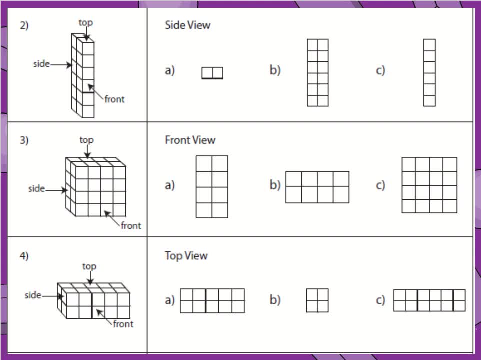 Okay, let us have a look at this one. So let us see what is the side view of these cubes or these 3D shape or object. So what does the side view look like? So we are looking for the side view. Does it look like this with two cubes? 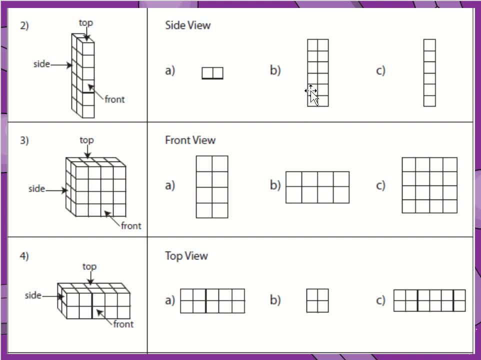 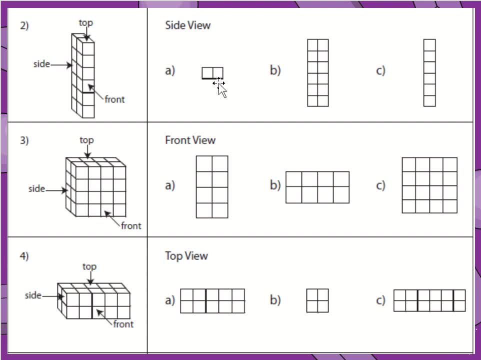 If we were looking at it from the top, it would be a triangle. If we were looking at it from the top, it would be a triangle. I reckon if we looked at it from the top, it would look like this. If we looked at it from the side, it would look like this. 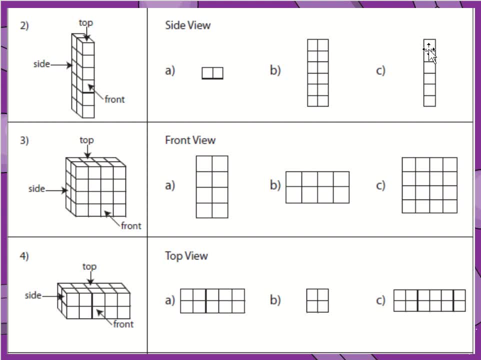 And if we looked at it from the front, we'd only see it from one column, So I would pick B. What about this one? Okay, we have to figure out what is the front view of this 3D object. Does it look like two columns? 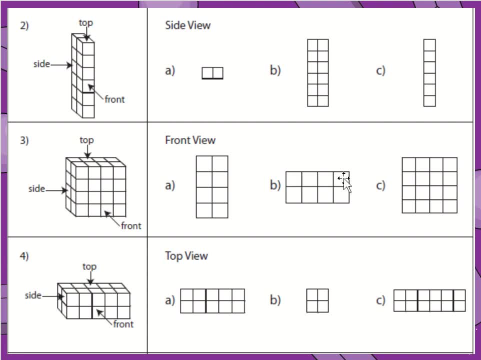 Does it look like four columns? Does it look more like a square? Now, I think this is the side view, This is probably the top view, And this is the front view. Now let's have a look at the number four, this one here. 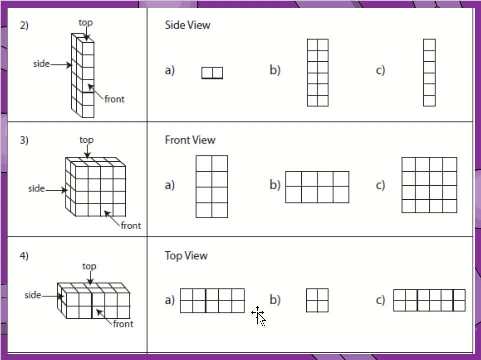 So what does it look like from the top? Does it look like A, B or C? Have a look. Now we should actually count the columns One, two, three, four, five. One, two, One, two, three, four, five, six. 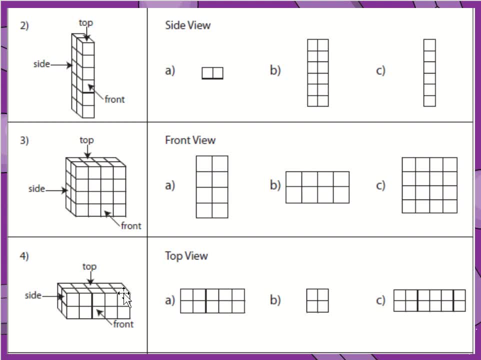 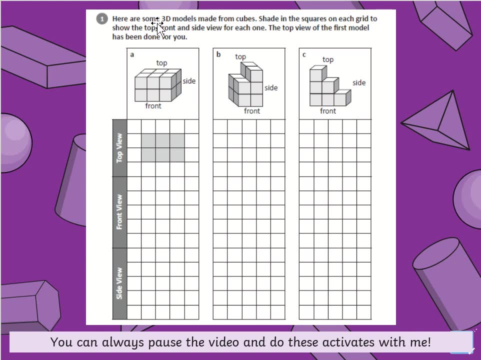 Let's count what it would be: One, two, three, four, five. So it would be A All right. This is what you are doing today. So here are some 3D modules made from cubes. Shade in the squares on each grid to show the top, front and side view for each one. 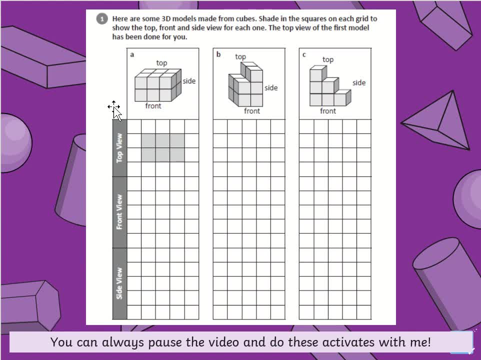 The top view of the first column. The first model has been done for you, So have a look at this model here. This is the top, This is the side, This is the front. So you will need to shade in and colour in. 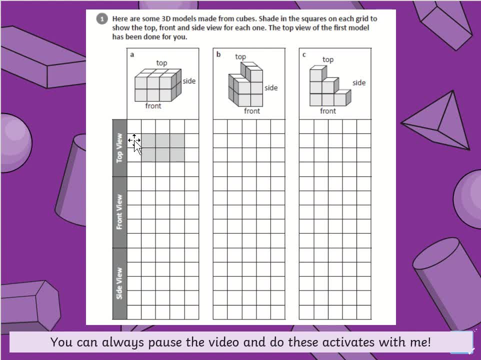 What does it look like? What does the shape look like? Okay, So this is the top view. So you can see that the top view has one, two, three, four, five, six squares, which is why they've coloured in one, two, three, four, five, six squares. 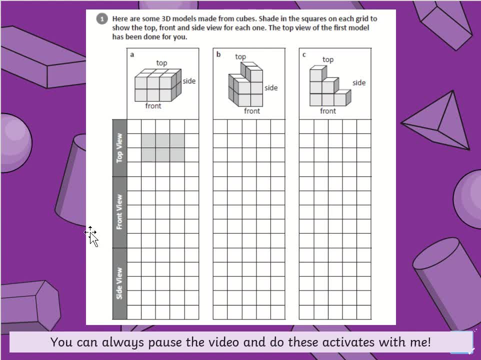 So three columns, two rows. If you have a look at the front view here, it looks the same. So you would colour in the same shapes. So I would colour in one, two, three across. one, two, three across. 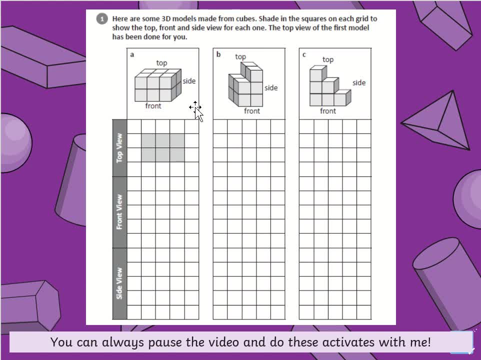 And that would be my front view, But the side view looks a little bit different, because there are one, two, three, four, Four squares that I would colour in and I would turn that into a square. So that's what I would draw. 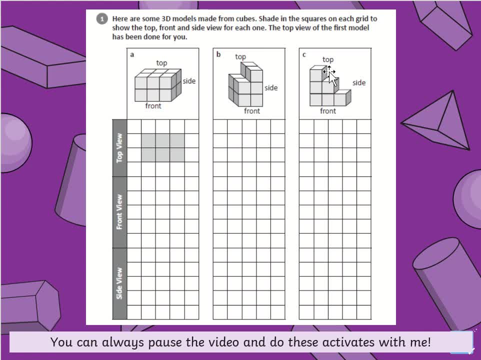 And then you do the same. You do the same thing with this for B and C. So you need to colour in and think about: what does it look like from the top, What does it look like from the front? What does it look like from the side?